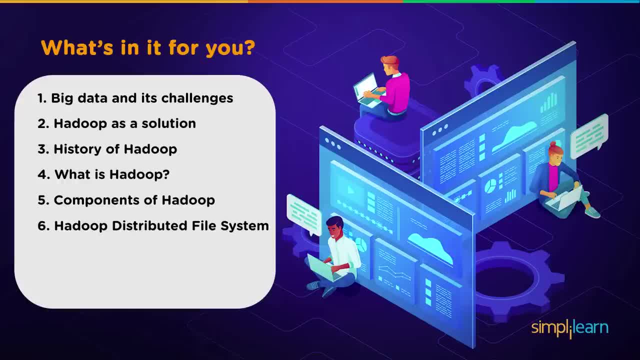 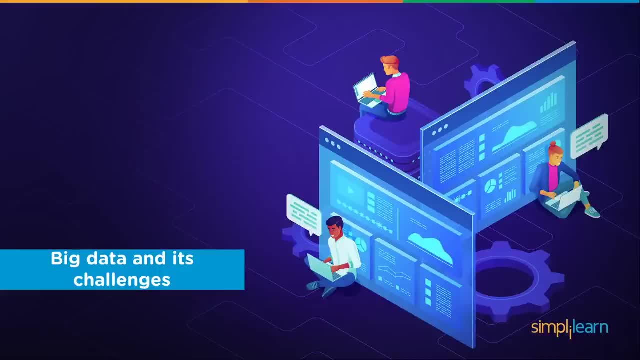 and then we'll dive into the components of Hadoop And we'll be looking at the Hadoop distributed file system, Hadoop MapReduce and Hadoop Yarn. So let us jump in and look at big data and its challenges. Data has evolved significantly over the last five years and 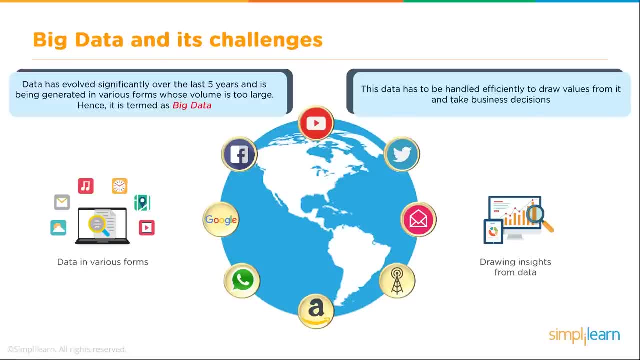 is being generated in various forms whose volume is too large, Hence it is termed as big data. In fact, this year alone, we probably generated more data than all the previous years added together, And we've generated just about any form you can think of Anything that's on your computer from. 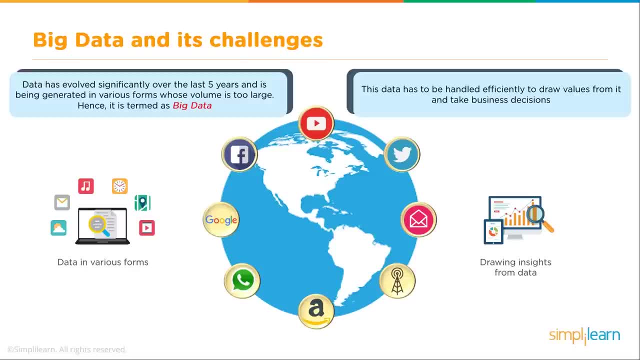 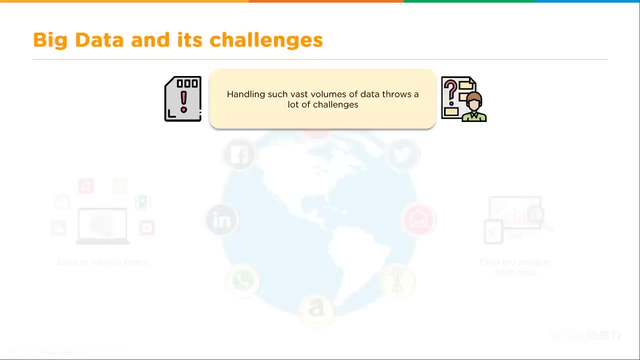 social media like Facebook, to YouTube, Email to locations and any of that- All those different forms of data- is just being massively produced. This data has to be handled efficiently to draw values from it and take business decisions. So when we talk about handling such vast volumes of data, it throws a lot of challenges at us. 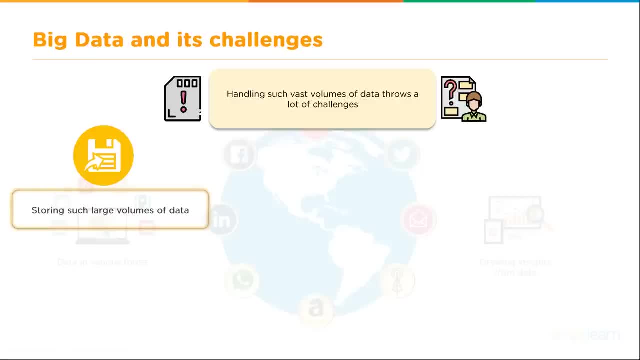 Storing such large volumes of data. Where the heck do we put it? Certainly, your personal desktop computer nowadays might have one, two or even 10 terabytes, But we're not talking 10 terabytes. we're talking petabytes and gigabytes. 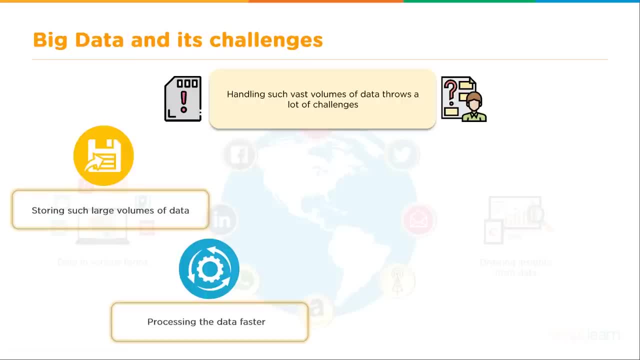 We're talking petabytes or larger, Processing the data faster. So we now have more things we can do to that data in different ways of processing it. How do we process it faster to draw those new predictions and understand what's going on so we can use that in our business Maintaining? 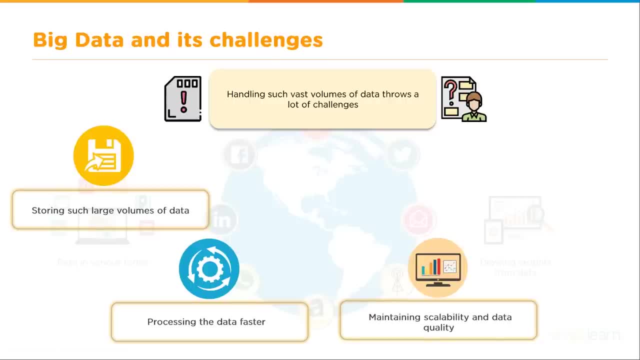 scalability and data quality. Now that's a tough one. How do you up your computer system so you have a bigger computer on your desk, or even a bigger computer than that, or a super cool machine? At what point can you no longer afford that? 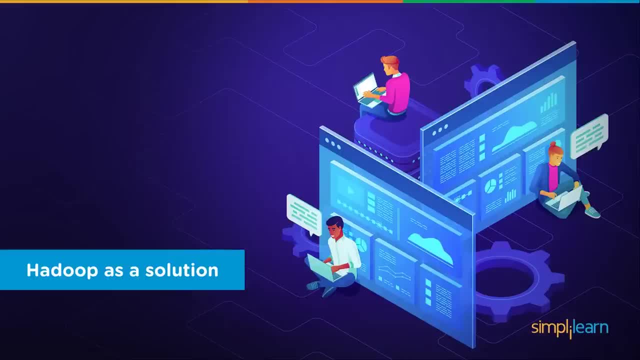 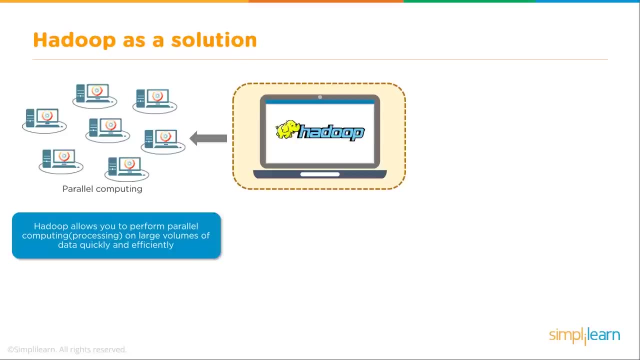 And keeping the data safe and secure. So Hadoop as a solution- And Hadoop is probably one of the biggest places in the market right now for storing and analyzing big data- So we talk about Hadoop as a solution. Its central is parallel computing And you can see we have the nice Hadoop elephant. 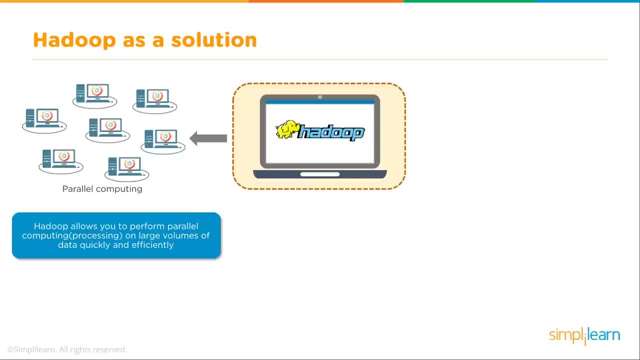 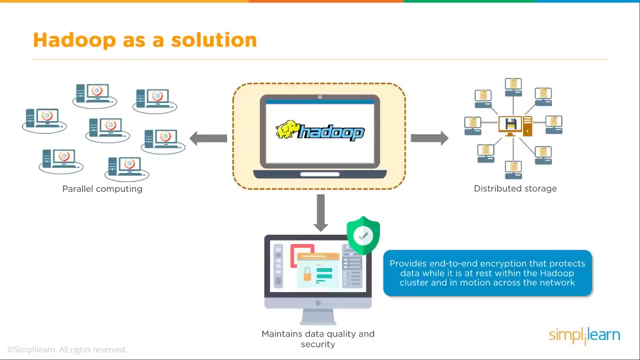 which is a symbol for Hadoop. Hadoop allows you to perform parallel computing or processing on large volumes of data quickly and efficiently. Hadoop stores data on multiple systems instead of on a single system. Hadoop provides end-to-end encryption that protects data while it is at rest within the Hadoop cluster and in motion across the network. 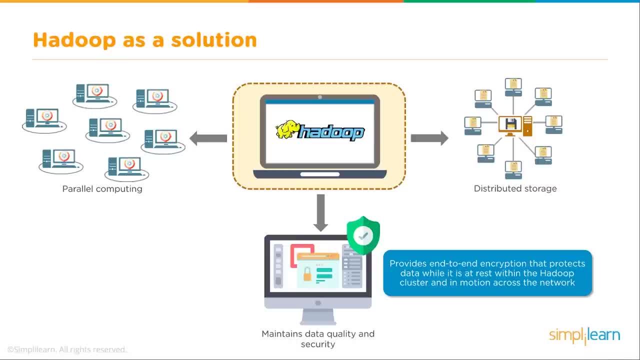 Now all of these sound like something simple, but it's actually a lot more complicated than you think. How can you do it affordably? Do you buy really high-end computers at $50,000 each, or enterprise machines? The bill for that grows exponentially. 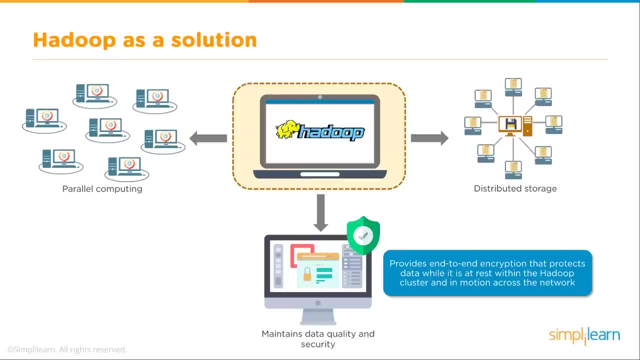 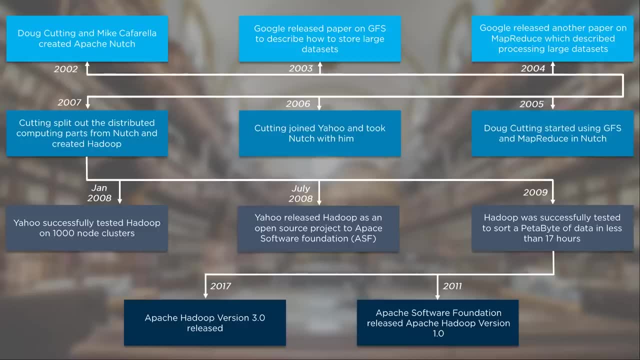 And so when we talk about what exactly is Hadoop, we'll see how that creates a solution that is financially doable by companies. Let's start with the history of Hadoop. We look at the history in 2002.. We have Doug Cutting and Mike Caffarella created Apache NUTCH. 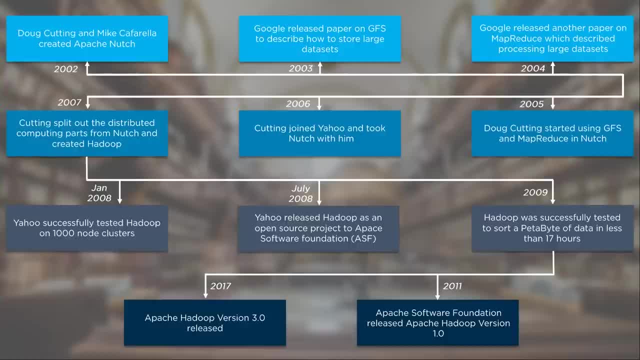 And in 2003,. Google releases a paper on GFS to describe how to storage large data sets. So Google on the back end is trying to figure out how can we efficiently and affordably store these data. Google released another paper on MapReduce, which described processing large data sets in 2004.. 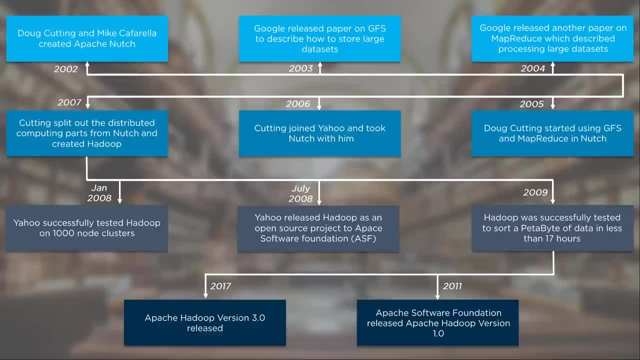 In 2005, Doug Cutting started using GFS and MapReduce and NUTCH. In 2006, Cutting joined Yahoo and took NUTCH with him, So now we have it going from the Google setup to under Yahoo, And in 2007, Cutting split out the distributed computing parts from NUTCH and created Hadoop. 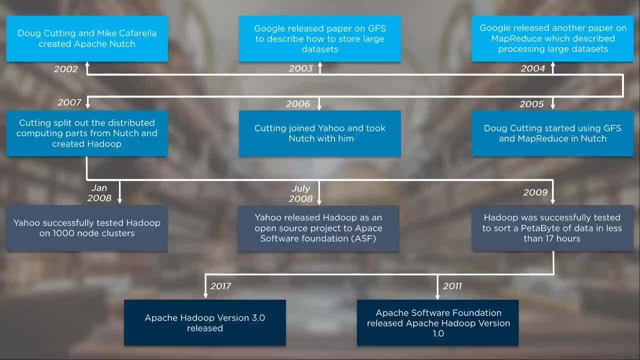 And that takes us into 2008,. January, the beginning. Yahoo successfully tested Hadoop on 1,000 node clusters: 1,000 computers that could handle processing the data in parallel and storing it in parallel. In July of 2008,, Yahoo released Hadoop as an open source software. 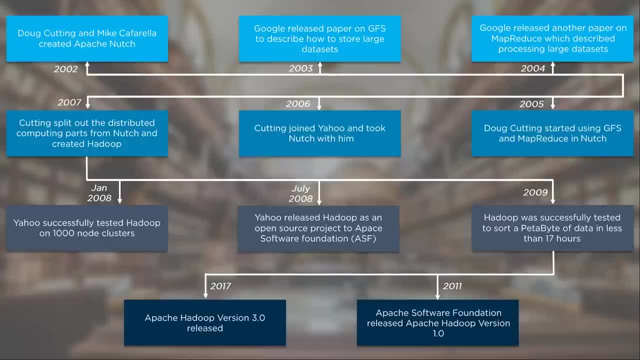 In July of 2008,, Yahoo released Hadoop as an open source software. In July of 2008,, Yahoo released Hadoop as an open source project to Apache Software Foundation or the ASF, And in 2009,, Hadoop was successfully tested to sort a petabyte of data in less than 17 hours. 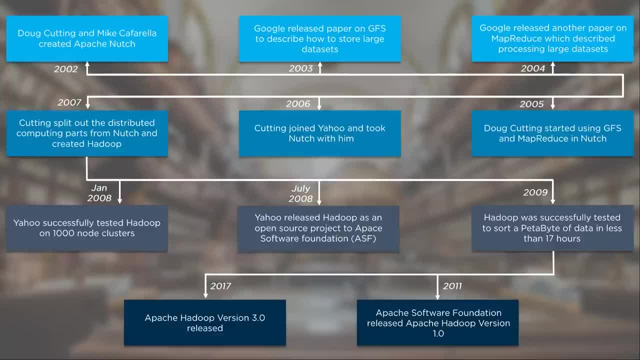 Now we think of 17 hours. we try to picture what a petabyte is. I have trouble processing or sorting through a whole terabyte of data in a few hours, you know, on my personal desktop. So we're talking a petabyte. 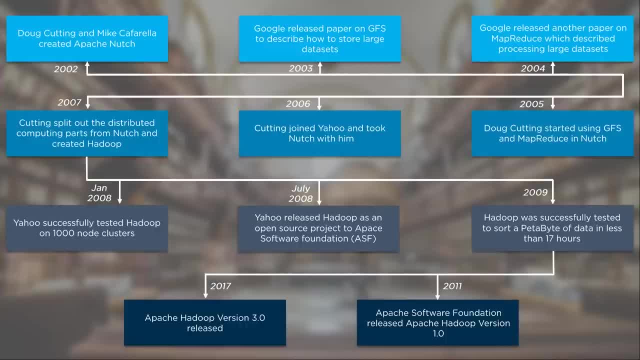 We're talking thousands of terabytes, And in 2009,. that was kind of when it was really mature. And then 2011,, Apache Software Foundation released Apache Hadoop version 1.0.. That brings us up to the last major release in 2017, which is the Apache Hadoop version 3.0. 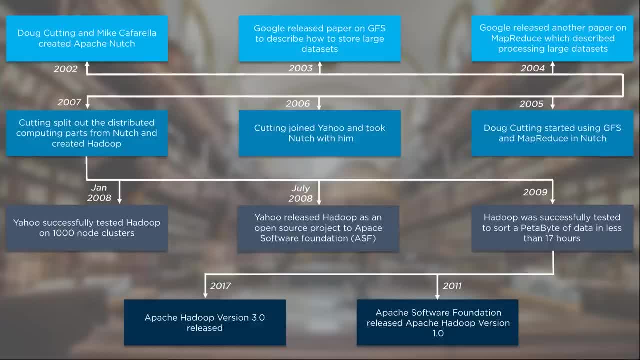 And if you were ever around in the 90s, you would know that any minor production of software releases was a significant turnaround And in large businesses- in fact I talked to hospital software- if you went back to the 90s, some of their databases took 10 years to evolve. 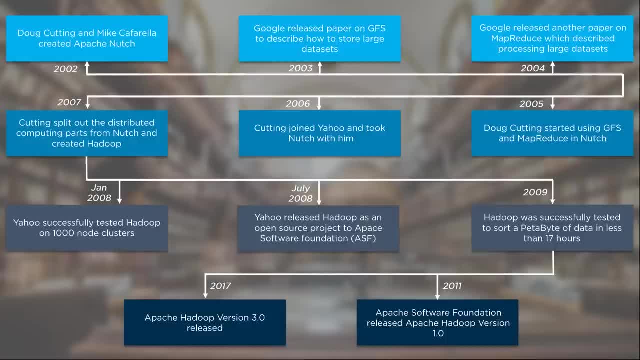 And so you look at this evolution Where we already have a release coming out, an open source, back in 2008,, July And it's pretty exciting- from 2008 to 2011, we already have a solid release. 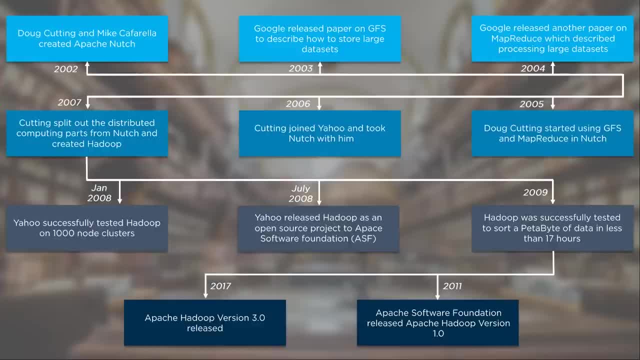 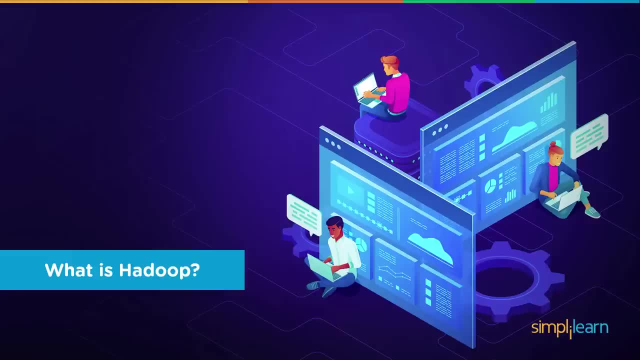 And then, from 2011,. over six years, we've had two major updates to version 3.0.. So that's going to lead us to the question: what is Hadoop? What exactly is this technology we're talking about for handling big data? 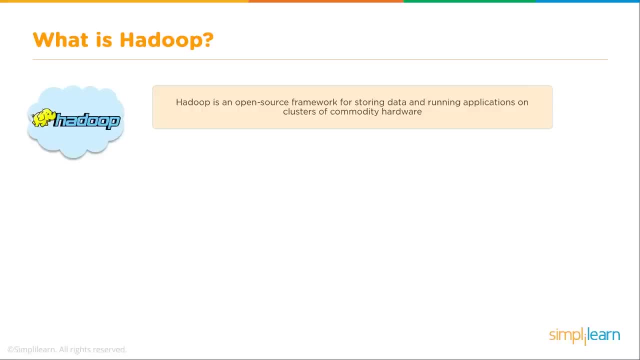 Hadoop is an open source framework for storing data and running applications on clusters of commodity hardware, And it's so key you can do it on commodity hardware, which is a tenth of the cost of enterprise machines. And so we look at this. we have our big data. 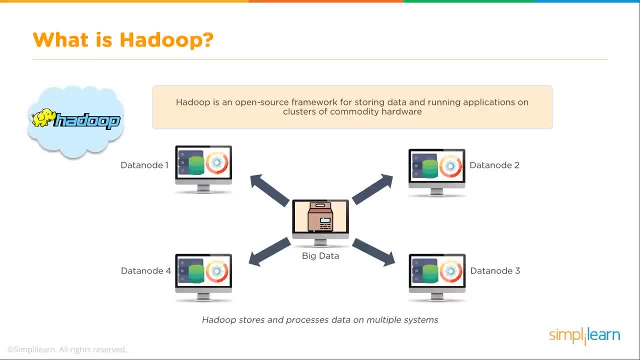 Hadoop stores a process data on multiple systems And you can see here we have data node one, two, three and four and they all are brought together to form big data. And each one of these machines- we talk about commodity machines- 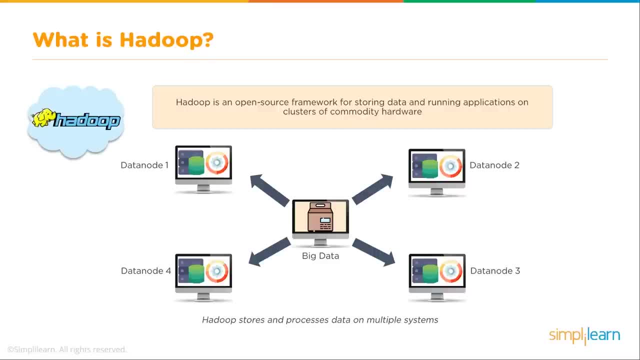 The best description I ever heard was a gentleman who works for- I guess I can't really say- the main company, one of the major companies out there, But he says: you know, these are your knockoff machines, These are your Chinese knockoffs. 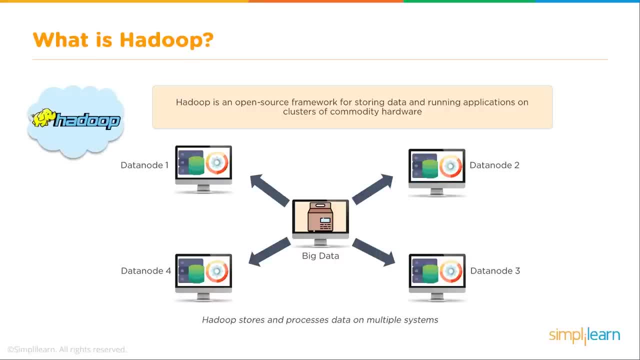 These are your ones that are brought in from other countries. You open a box of commodity computers and they're going to work, But you'll probably have like one in 20 that goes out early because it's not a solid machine, It's not an enterprise machine. 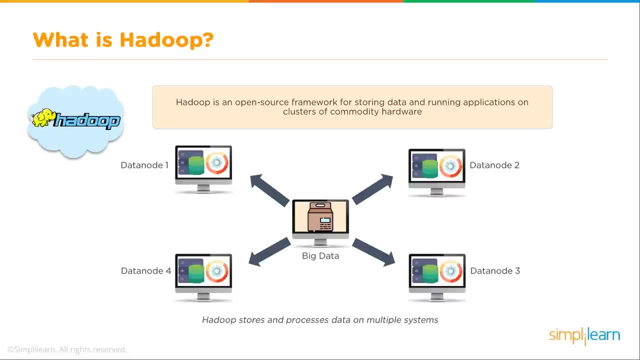 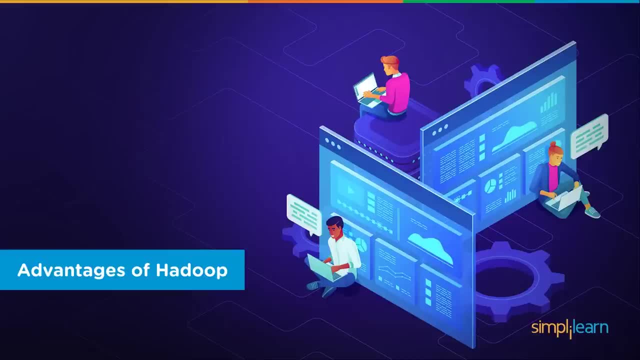 So it's not as high quality as the enterprise machines, But with Hadoop we can use commodity machines, and in such a way that it still holds the integrity of the data. So let's take a look at the advantages of Hadoop. I sort of listed one there as far as commodity versus enterprise machine. 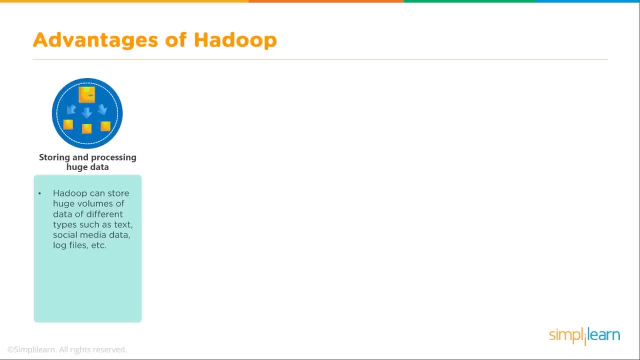 And the advantages of it. When we talk about advantages of Hadoop storing and processing huge data, Hadoop can store huge volumes of data of different types, such as text, social media data, log files, et cetera. Anything you can put on your PC, that's data. 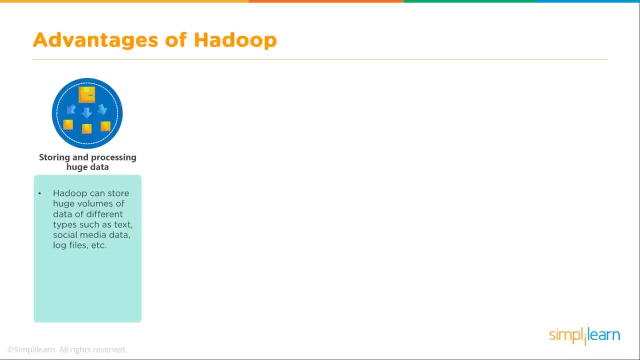 It's a file system. This is very different than, say, a SQL server which stores columns and rows and you have databases. Very different than a NoSQL server that only stores families of data and links them together. This can store either one of those. 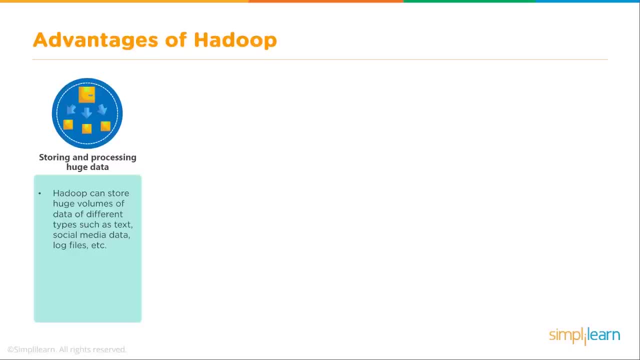 This can store just text documents. It's whatever you want to put on it, just like you can put it on your own personal computer. The computing power Hadoop's distributed computing model processes big data fast. The more computing nodes you use, the more processing power you have. 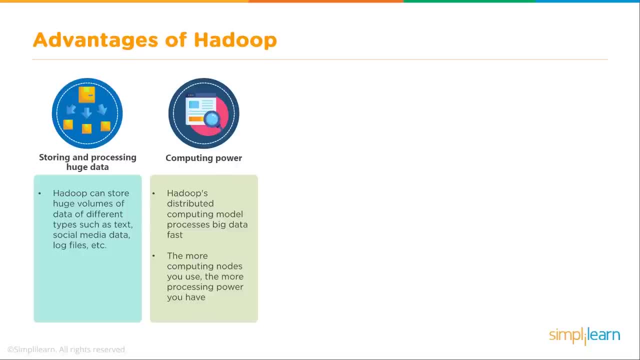 Now, obviously there's a little play here, in that if you have a lot of computers with high RAM and high processors on there, they're still going to each process more efficiently, And there's even ways to bring that up. We'll talk a little bit about the Hadoop ecosystem. 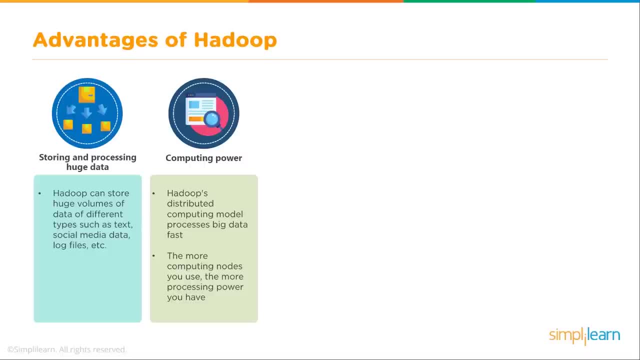 And how Spark can sit on top of that and it runs faster because it runs everything in memory, Where the Hadoop writes it to the disk and reads it up. We'll talk about that in just a minute, But let it know, the advantages of Hadoop is the computing power and the ability to store huge amounts of data. 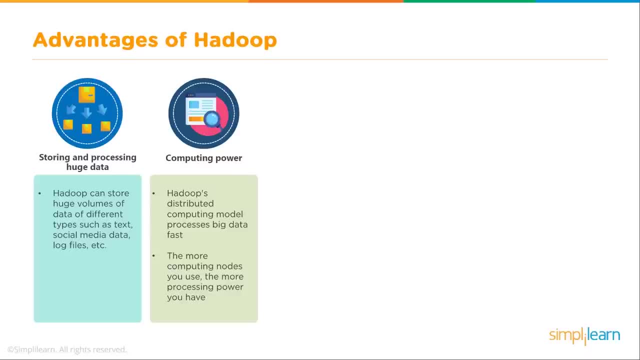 Those are the primary two things that it does, and a variety of data, And it's flexible. Unlike traditional relational databases like SQL Server or NoSQL Server, you don't have to pre-process data before storing it. You can store as much data as you want. 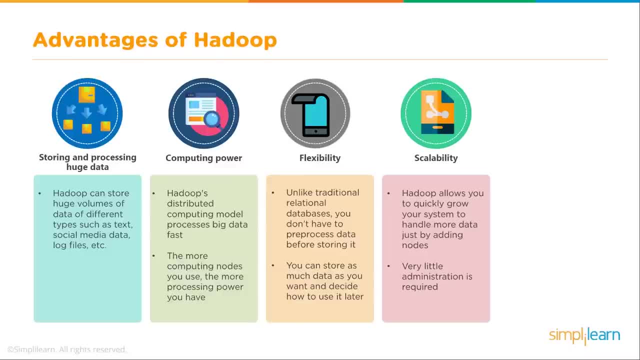 And decide how to use it later. It's scalable. Scalability is huge. Hadoop allows you to quickly grow your system to handle more data just by adding nodes. Remember I talked about commodity machines. Now, in most Hadoop clusters you usually have two enterprise computers for your masters. 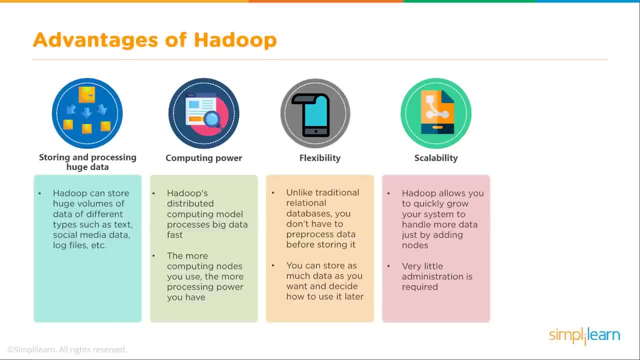 And then the rest are really affordable machines you can put on there And it has its own backup system and everything else, So that as you grow your Hadoop system and you add new racks on and new servers on, you're paying a linear increase in your data. 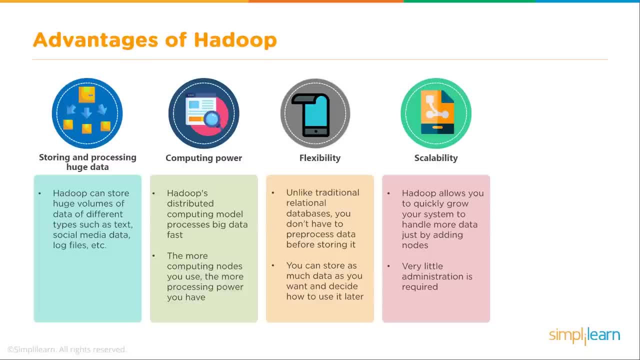 It's not going up exponential like you'd expect by going from a regular server into a Cray server Where suddenly you're paying a huge amount of money for a liquid nitrogen-cooled computer to handle the larger data. You're just adding one machine on each time. 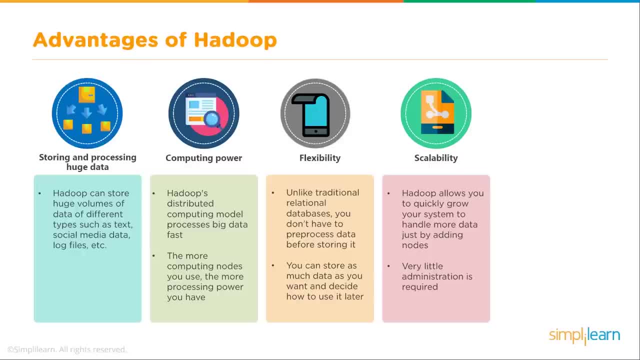 There's also very little administration. This one I love. There's very little administration required, So each computer is very easy to add in once you have your system going. Fault tolerance, Data is protected against hardware failure, And this is central to what makes Hadoop work. 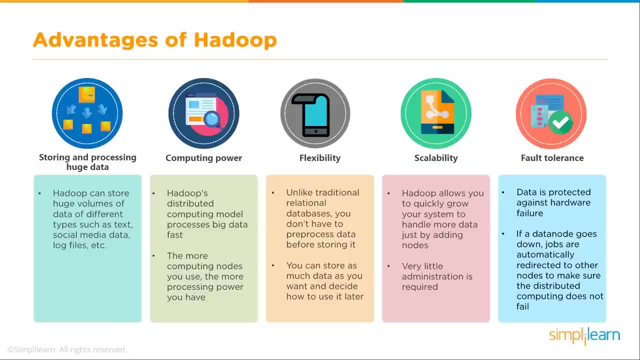 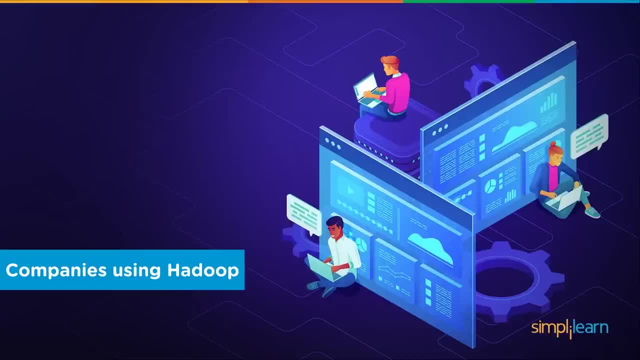 One computer goes down and the system doesn't care. If a data node goes down, jobs are automatically redirected to other nodes to make sure the distributed computing does not fail. So let's take a look at some of the companies using Hadoop. So you know where you're going with this as you dive into the Hadoop and big data. 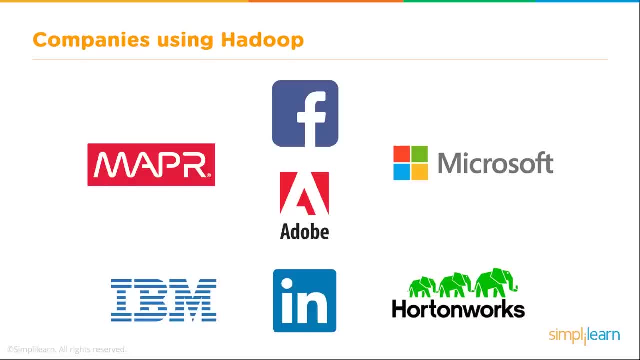 When we talk about the companies using Hadoop, we can look at Facebook, Adobe, Microsoft, Hortonworks, LinkedIn, IBM. Obviously, Google is using this. It's so widely used that it is now It's an Apache, open source, and yet Microsoft is now using it as one of their main backend frameworks. 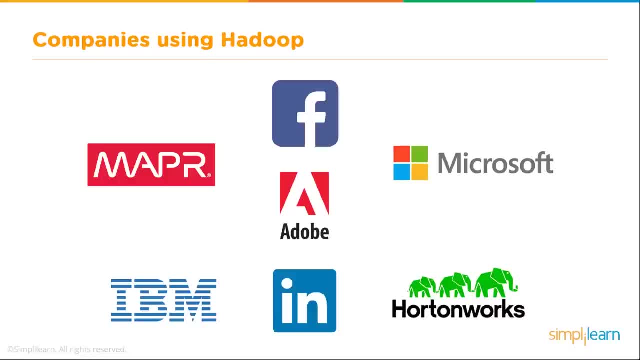 Hortonworks and Cloudera, which isn't listed here. those are both packages that specialize just in the big data and helping companies and support them, So it's really widespread. It's becoming just a very common setup to see in most large business industry. 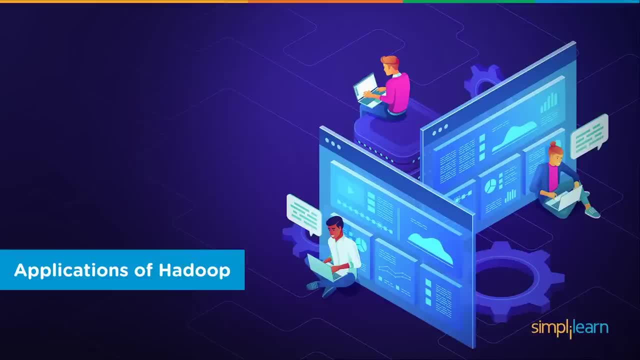 Let's take a look at some of the applications of Hadoop, And these are almost endless. Any place you have a lot of data or a lot of process. It's a lot of data, It's a lot of processes. It's a lot of data. 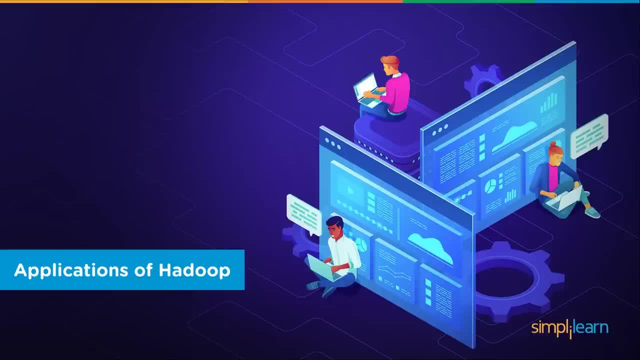 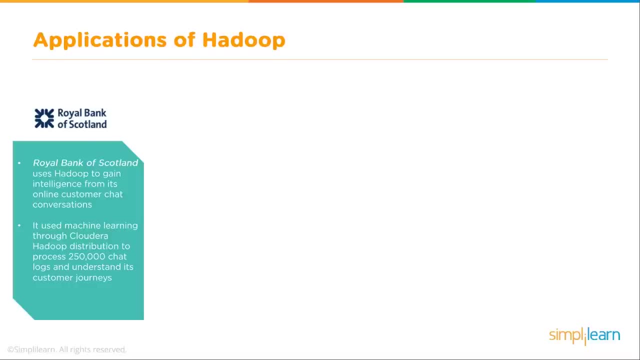 You could have a small amount of data and have a huge amount of processing on that data. That's a place you're going to start seeing Hadoop and or Spark, which sits on top of Hadoop. So we look at the Royal Bank of Scotland. 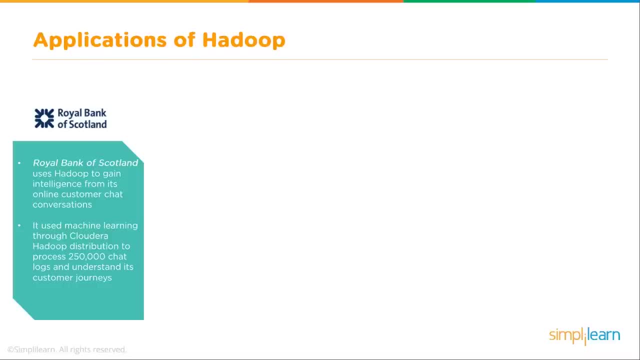 Royal Bank of Scotland uses Hadoop to gain intelligence from its online customer chat conversation. It used machine learning through Cloudera Hadoop distribution to process 250,000 chat logs and understand its customer journeys. And I mean that's just one bank. 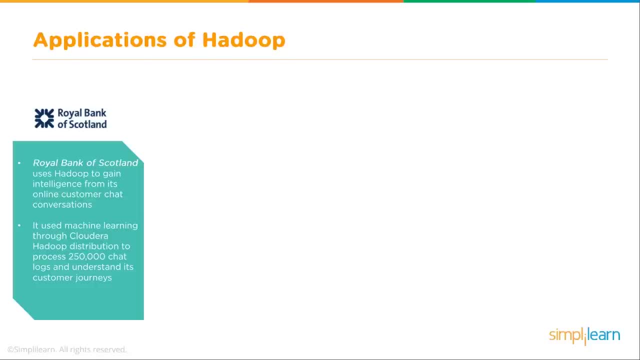 It is so common in the banking industry. now that it's, I would say, most large banks probably have some form of Hadoop file system somewhere so they can properly analyze their data. M&S, Marks and Spencer uses Hadoop to analyze its data from multiple sources to understand its customer behavior better. 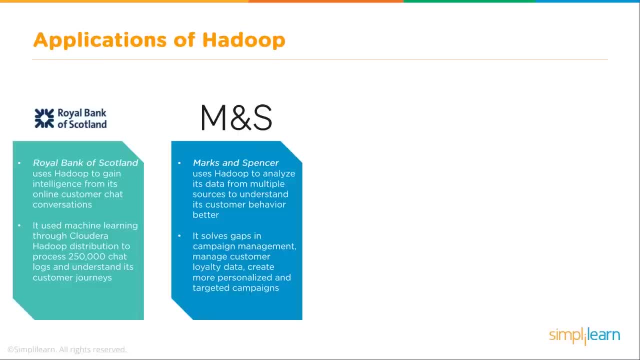 It solves gaps in campaign management, manage customer loyalty data, create more personalized and targeted campaigns. And we have the Royal Mail. Royal Mail is a British postal service company that uses Hadoop to transform the way it managed data across the organization. It can now identify: 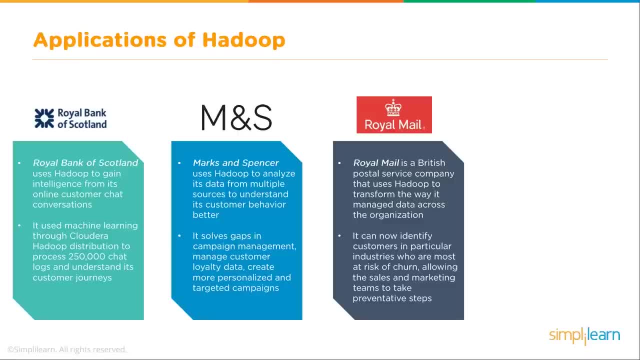 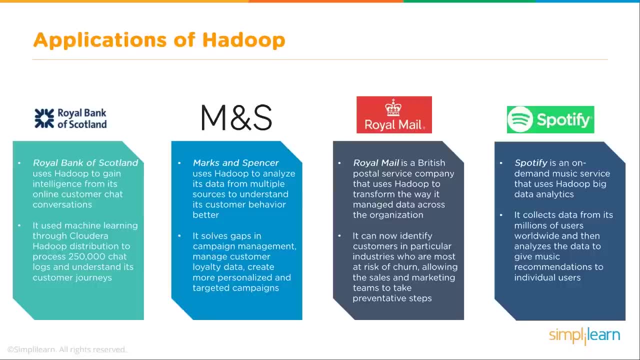 Customers, in particular, industries who are most at risk of churn, allowing the sales and marketing teams to take preventative steps. and Spotify. Spotify is an on demand music service that uses Hadoop big data analytics. It collects data from its millions of users worldwide and then analyze the data to give music recommendations to individual users. 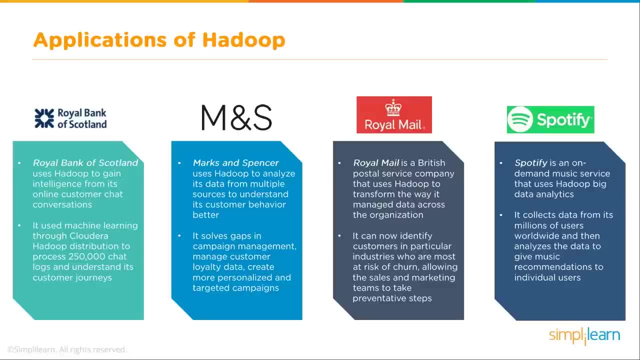 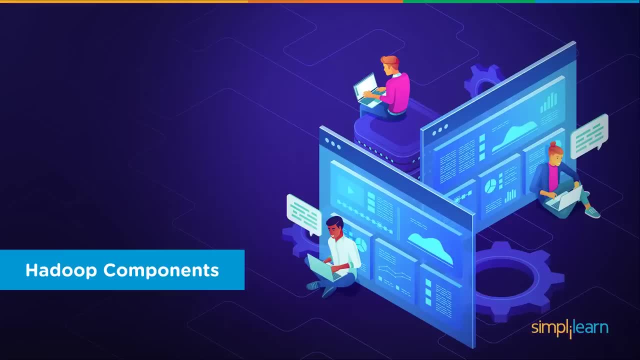 So here's just a couple examples of some of the applications of Hadoop right now in the market, and it goes way beyond this. So let's dive in and see what really is Hadoop's about and let's look at the components of Hadoop and we're going to talk a little bit. 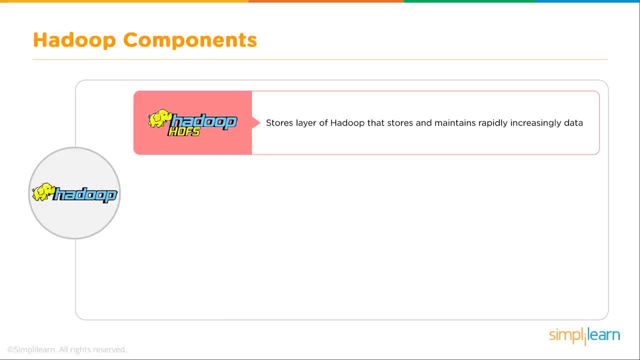 What exactly is Hadoop? We'll start with the components. when we talk about Hadoop components, We usually start with the HDFS, Hadoop, HDFS or the Hadoop file system, and you can think of that very much like your computer file system. 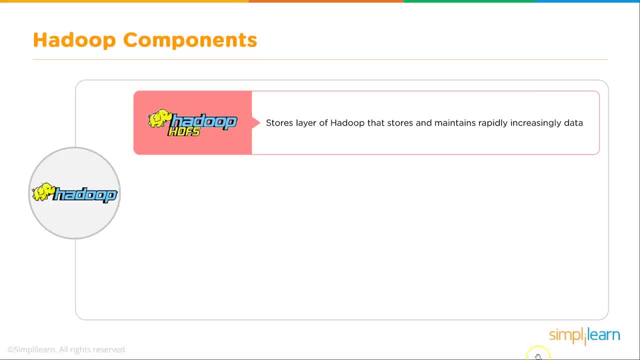 You have folders, you have There's a lot of different options in there, but you can store just about any data that you want into the Hadoop file system. And then there's a processing, the processing layer. We have a dupe that perform parallel computing of data, and we talk about map reduce. 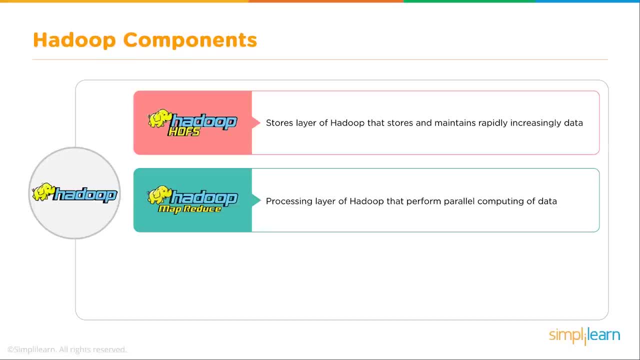 And nowadays in the industry of data analytics there is a specific process called map reduce. But when you get into programming you need to go beyond that particular system because a lot of different options with Hadoop and think map reduce. It's so important. 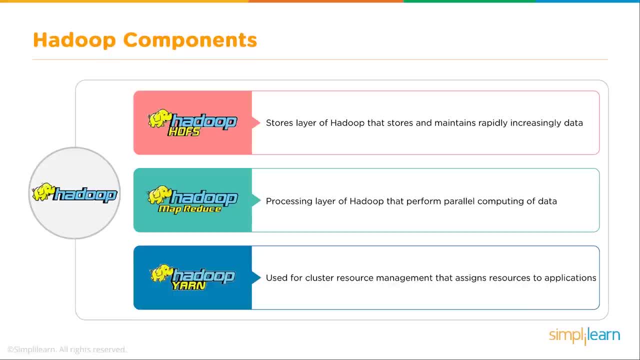 And then there's yarn. This is used for cluster resource management. that assigns resources to applications, And yarn stands for yet another resource negotiator. This is what makes it work across the different machines and tracks it all down. So we look and we're going to dig in deeper into each of those. 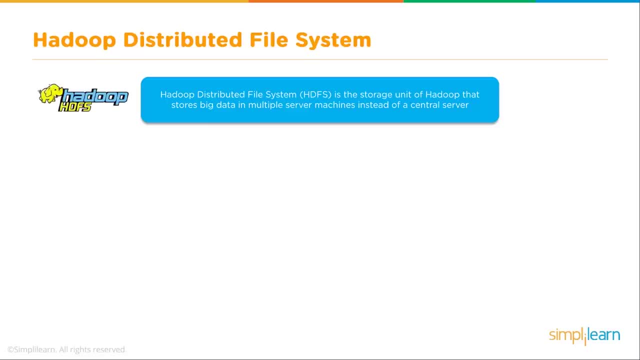 And let's look at the Hadoop distributed file system. So we talk about the Hadoop distributed file system, or the HDFS. It is the storage unit of Hadoop that stores big data in multiple server machines instead of a central server, And this is huge. 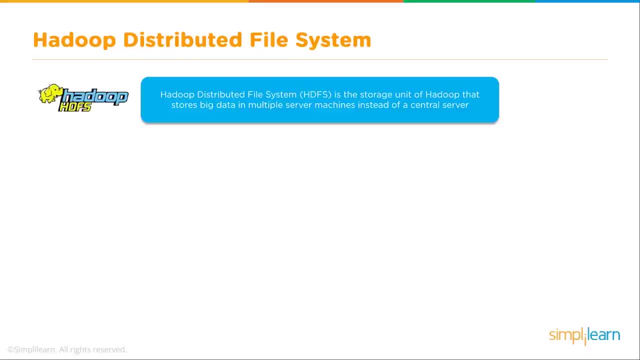 I talked about that earlier. Instead of upgrading to a really expensive Cray machine, they use liquid. I think that some of the new ones that they put out actually use liquid oxygen To cool them, Or liquid nitrogen, And they're these massive machines. 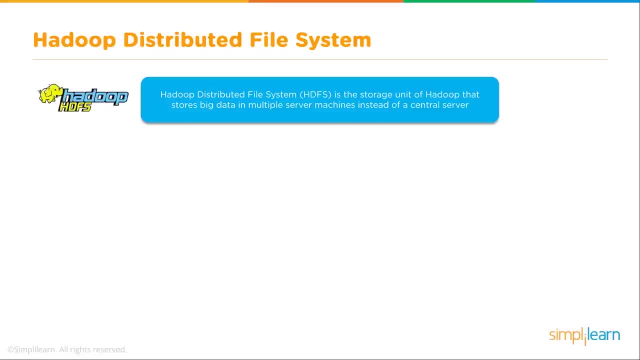 And they're great, But they are so expensive. They run millions of dollars just to maintain them, And we're not even talking about the cost of buying it and setting it up. So we look at this, We want to get away from that. 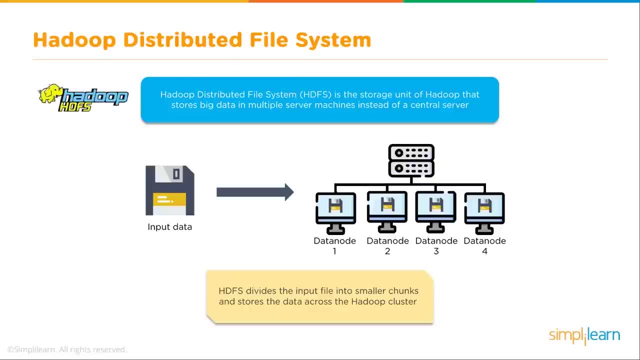 How do we get away from one huge, expensive machine? Well, we have our HDFS And it divides the input file into smaller chunks and stores the data across the Hadoop cluster. And you can see, here we have our input data And then we have our different data nodes. 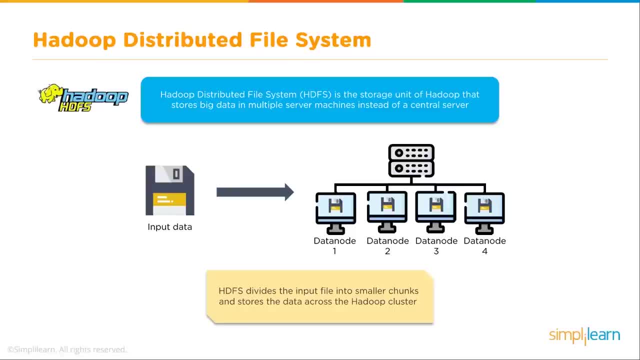 And usually you have at least ten data nodes in a cluster. And then they have the two computers on top which I talked about, Which usually are the enterprise machines, since they're the master ones, And we'll talk a little bit more about those. 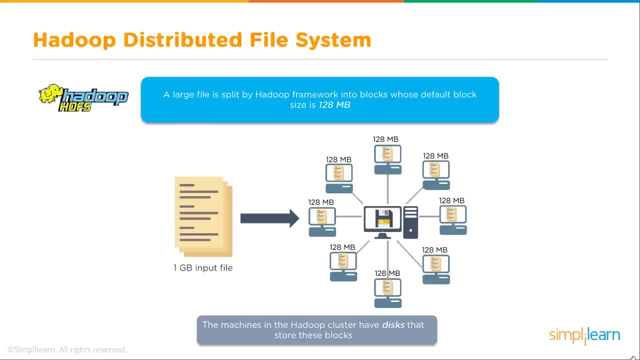 So you have your data comes in. It's going to distribute it across all the different nodes. The large file is split by Hadoop framework into blocks whose default block size is 128 megabytes, And this has changed over time. The original one was 64 megabytes. 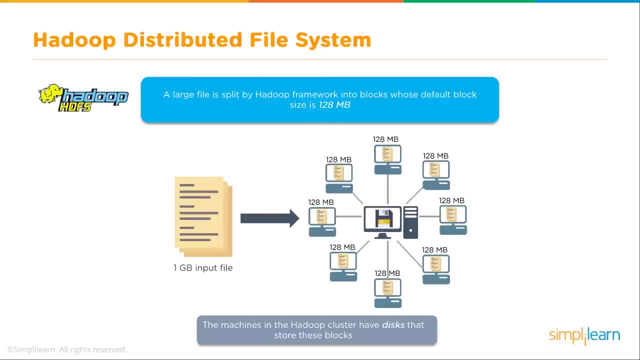 And although there's reasons to switch it on the size, depending on what it is you're storing and why, Generally 128 megabytes Is a good size for most of the stuff you're going to work with. So you can look at here we have a one gigabyte input file. 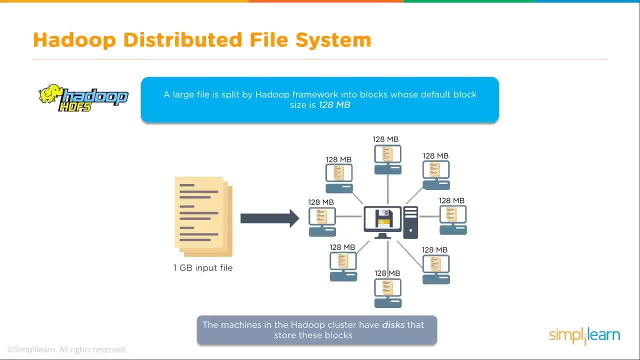 And you can see how it's split it up to all these different nodes. The machines in the Hadoop cluster have disks that store these blocks, So, just like they have a hard drive, It might be a solid state drive, depending on what kind of setup you're looking for. 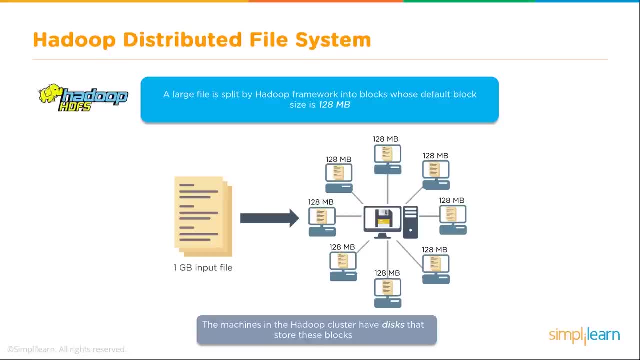 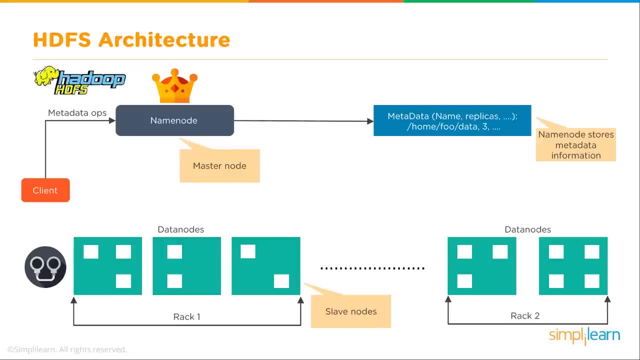 But, just like your computer is storing this data in these different blocks, Instead of it being on one hard drive, it's distributed across all these different machines, And so we look at the full HDFS architecture. We come in here, We have our client machine. 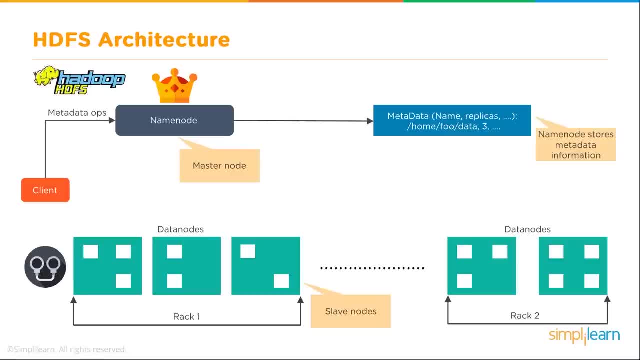 That's you working on your computer, typing away. You put in your data and you're sending it up. We have our metadata ops And that goes into the name node Or the master node, And this is going to be an enterprise computer. 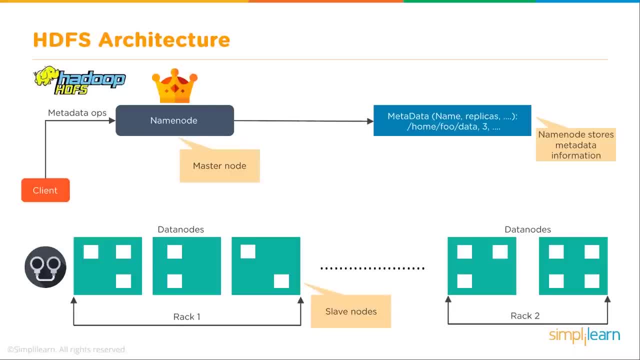 That's your point of failure. So you want that to be a solid computer. One of the points of failure. And that creates the metadata Names replicas. You can see here we have home food data. So the name node stores metadata information. 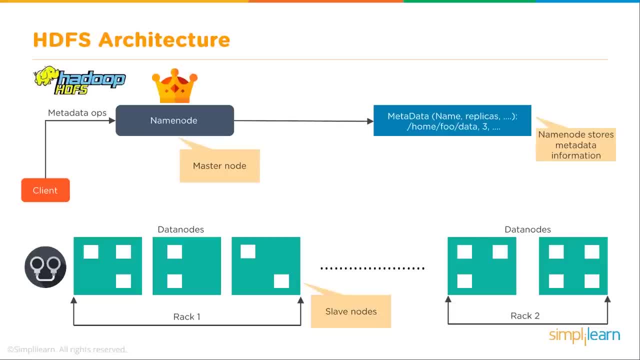 It tells it where it is. And then you have your slave nodes. And your slave nodes, we have like rack one and rack two And you'll have your data nodes down there. Those are all slave nodes. So these are racks of servers that you've installed. 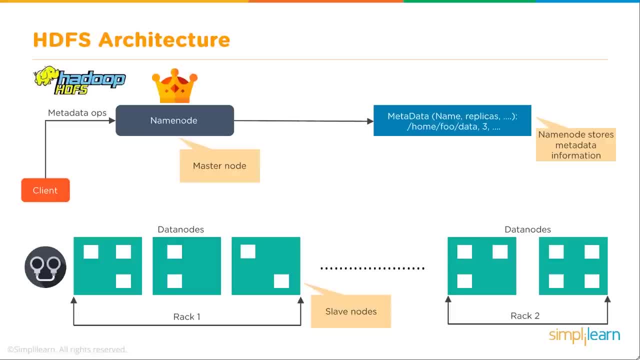 And if you remember I mentioned these are the cheaper computers. These are about a tenth of the price of an enterprise server. So we're looking at a tenth of the price for each one of these servers on the rack And usually you run the racks are all going to be in one room. 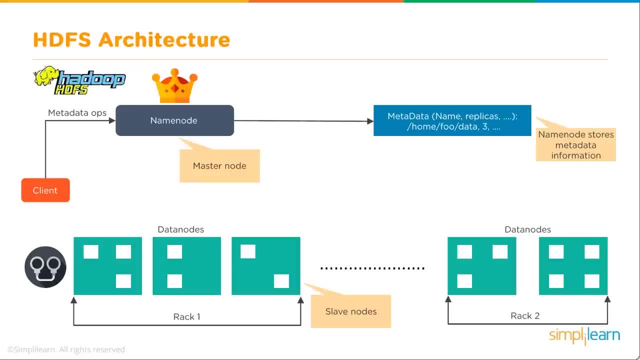 Because they've got to talk to each other very quickly. You usually don't have them spread out into different areas, Except for very special setups. So for the most part you're talking about this room full of servers and racks of servers, And a client can read data from the data node by consulting the name nodes. 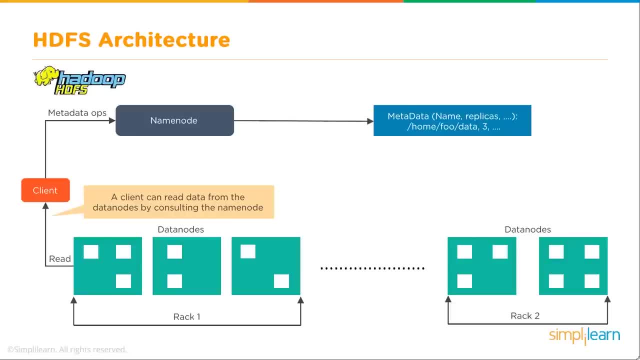 So it goes up to the name node and says hey, where's my data? And it says here's the data nodes, And then the data node sends the data directly back to the client. That would be you on the computer looking something up. Client can write data to the respective data nodes. 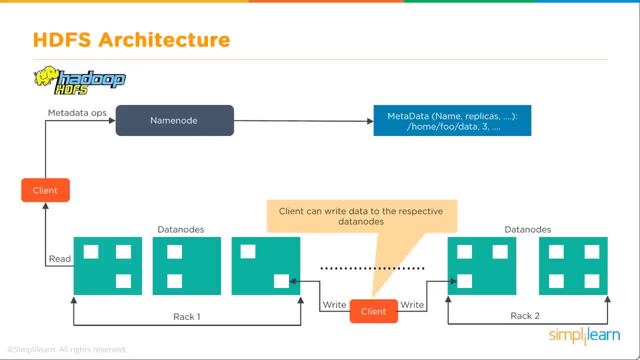 So it's in the same way. the client looks at the name node And the name node says, hey, this is where your data is going to go. And then the client writes it up to the server or whatever setup. it tells it it's going to put that data at. 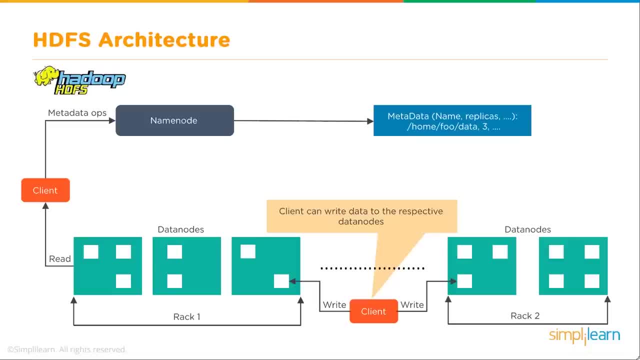 And when you're looking at Hadoop, you're only seeing one huge data file system. You don't really, as a programmer, know where the data is. Now, as an admin, you might track that down to see what's going on And make sure your servers aren't going down. 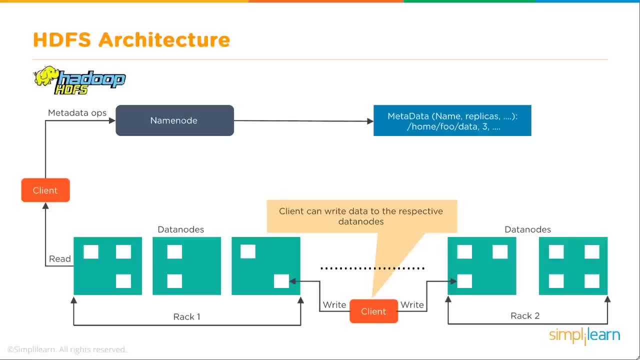 But as a client it sees all those different slave nodes or data nodes as one single file system. The HDFS allows you to perform block operation and replication of data blocks to different data nodes. So let's dive into Hadoop MapReduce. So the Hadoop MapReduce. 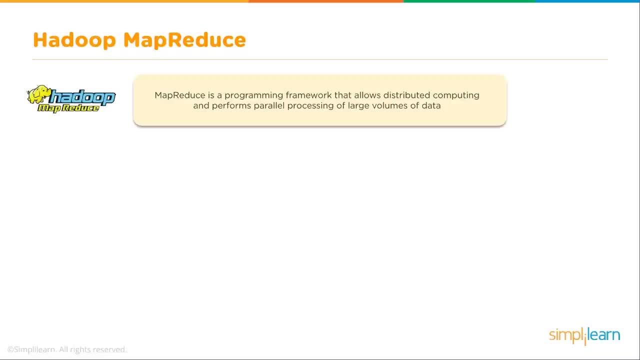 MapReduce is a programming framework that allows distributed computing and performs parallel processing of large volumes of data, And so we can see here: we have our master node in the middle, which is telling where everything goes and where it's at, And then you have your slave nodes on the end. 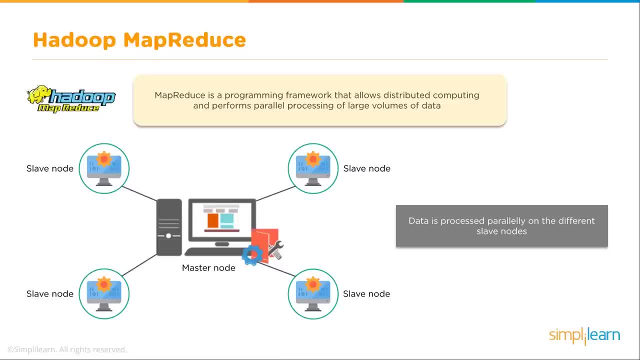 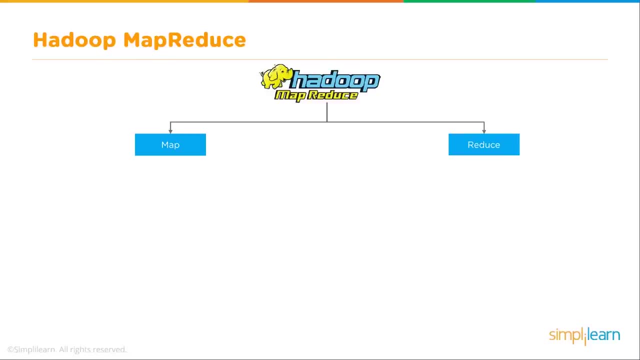 And data is processed parallelly on the different slave nodes And the way that looks is we have. this is so important If you're doing any kind of programming in big data. This understanding this little basic setup here is so important to think MapReduce. 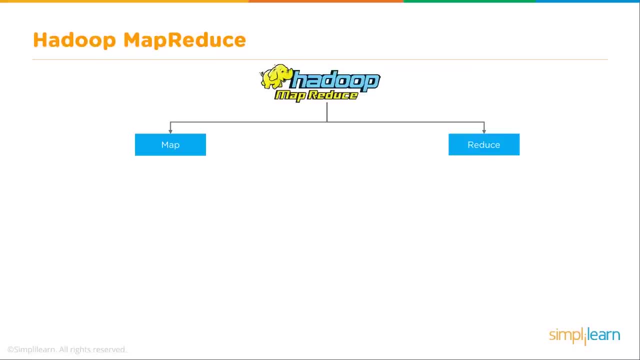 Even if you don't use a Hadoop MapReduce system and you use a different system on top of it, You still need to be able to think: MapReduce And we look at map. We have our input And we map tasks. We have our mapping process. 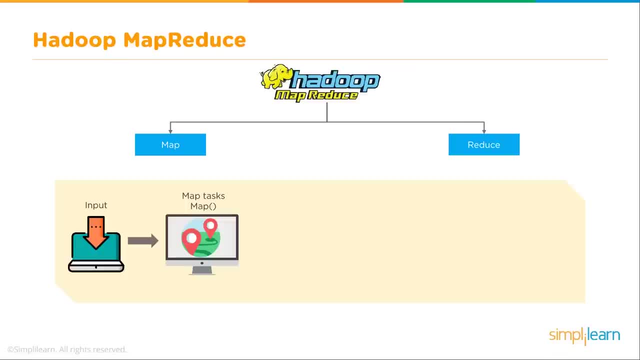 Now think about this: When we do a map process, It has to be anything you can do on a single piece of the data. What is a map? What does that mean? Well, that means if you have- let's look at- a standard SQL Server database. 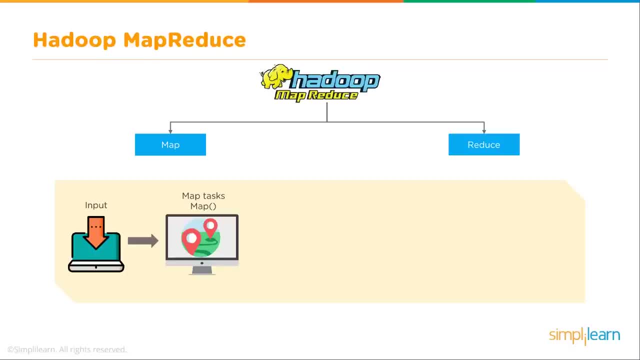 Because you can store SQL data in Hadoop. So if you're looking at that each row, you want to do a process on there. So if you have, like the user's name, their age, how many cells they did and something else, 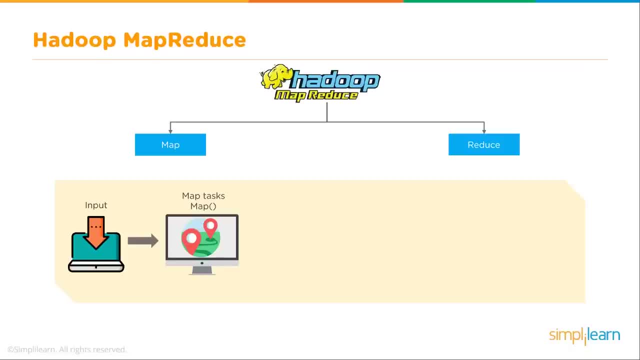 Any computation that uses just that data in that row would be in your map task. If you're processing documents, You might have a document that opens up where you're doing word count And it does all of the mapping processes on that one document. 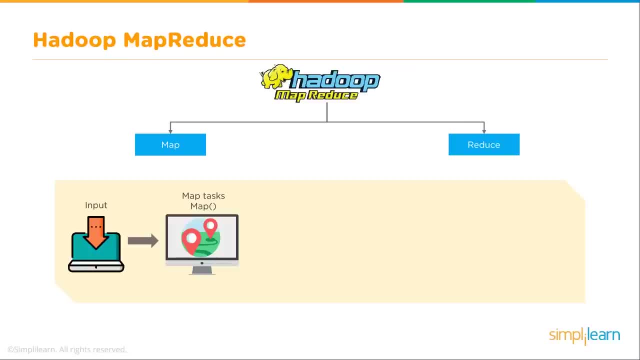 We're not comparing it to the other documents yet. We're just looking at that one document. We're counting how many words, How many positive words, How many times did they use the word cell, Close the cell, Finish the cell? Maybe you're looking at a terrorist block. 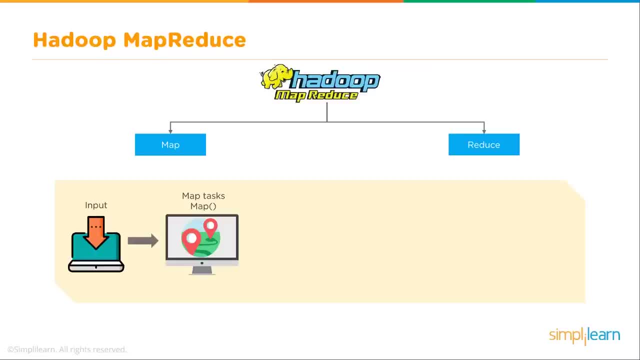 How many times did they use in the Twitter account some kind of reference to violence and things blowing up? Maybe you're looking to find out what products they like. How many times did they have a positive reference for the product Good, Whatever Good. 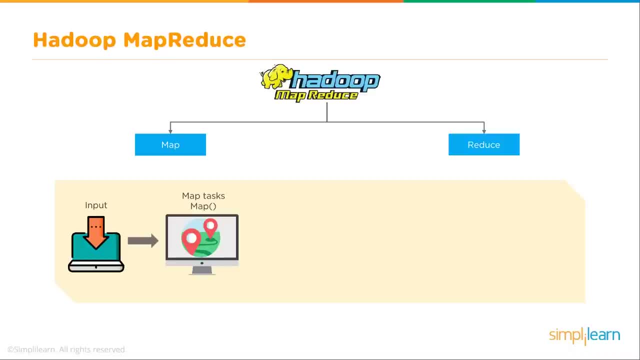 Excitement. That was cool, That was nice. So we're counting words in that tweet, In that document, In that row of the database. That's what we mean by mapping. Whatever you can do on that, one object is done on mapping. 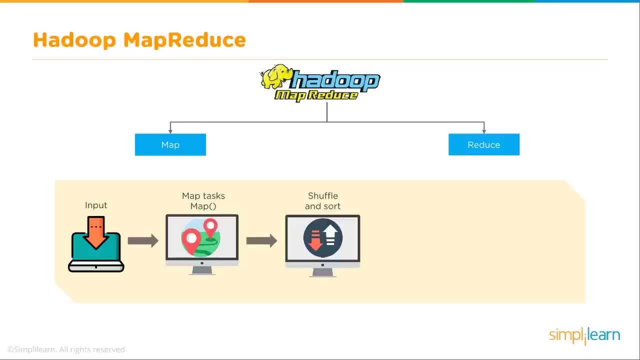 And then the computer does this on the back end, It does a shuffle and sort. So now we're going to group things together. Then we start to add stuff together, Like: how many times in all your documents did you use the word deception? 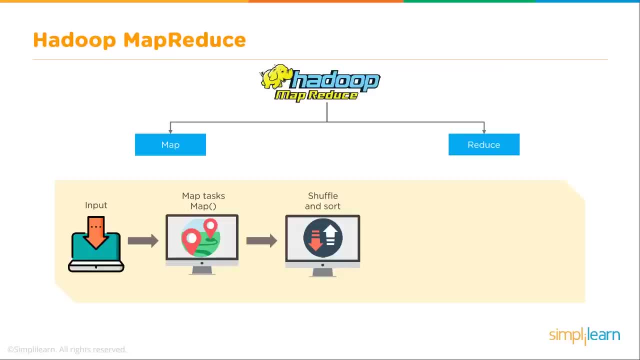 Maybe it's a political analysis. Maybe I'm getting myself in danger there Discussing politics. You're analyzing all these documents and you want to know how many times was the word deception used Or how many times was the word economic and growth used in the same document together. 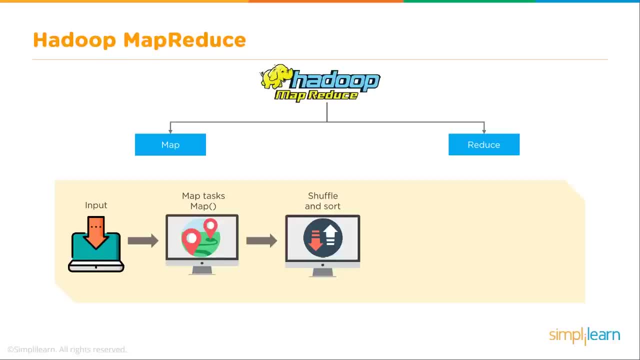 In that you want to buy, or two words together, So economic growth. So you might count out all the times it was used in all the documents And then you might find out which documents had the most references with economic growth. And then you start getting a count and a weight on those documents. 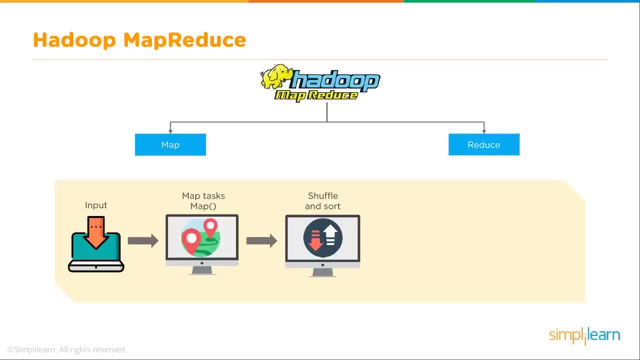 So we're going to shuffle those numbers and sort those numbers together. We get the individual documents And then we shuffle just the deception into one group And we shuffle just the count of economic growth into one group, And then we get to the reduce task. 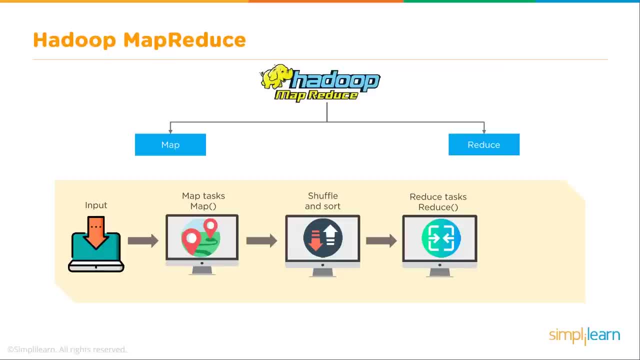 And the reduce task would be for each document. It might be: how many times was the word economic growth used And how many documents was it used in? We're going to reduce that down to something you can look at And you can see here where you might map, shuffle and sort. 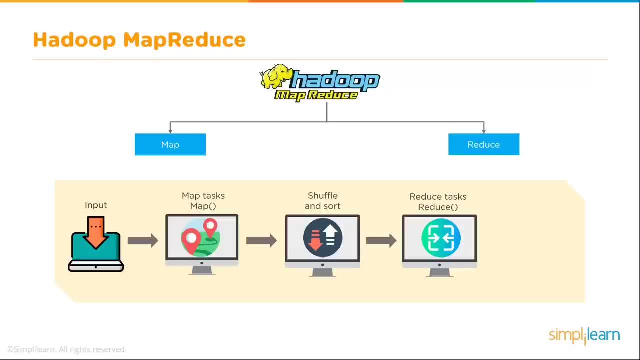 You might map again, Shuffle and sort, Reduce. You can end up with a very lengthy pipeline here as you try to get to the answer you want. So it might be when you look at averages and things like that. Again you want to think: what can I do to one piece of data? 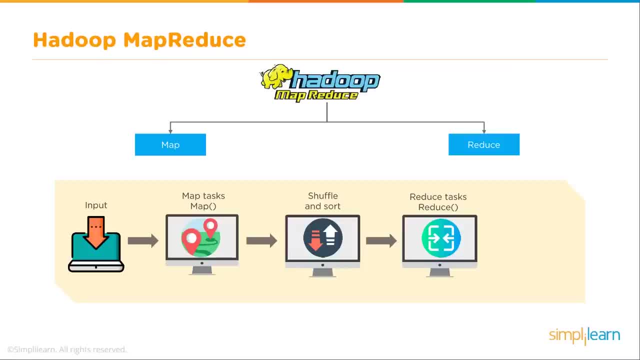 And then I want to shuffle it around, And then I want to reduce that to something I can see as a human being. I don't need thousands of numbers, I just need the top numbers that say these top three documents have the most positive outlook for economic growth. 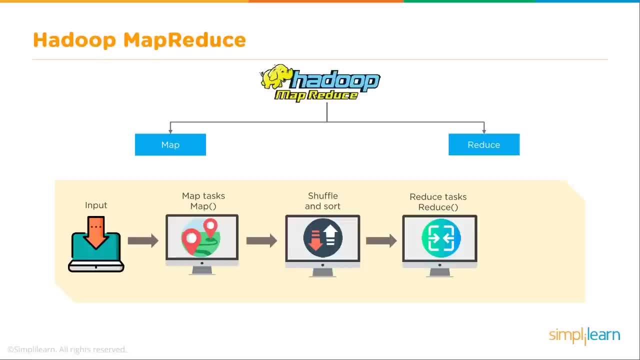 According to Twitter feeds. So these are what people are interested in. I want to reduce that down to what I can read And map reduce Again. you want to think: map reduce And then map reduce in. Hadoop is an actual process, A Java process. 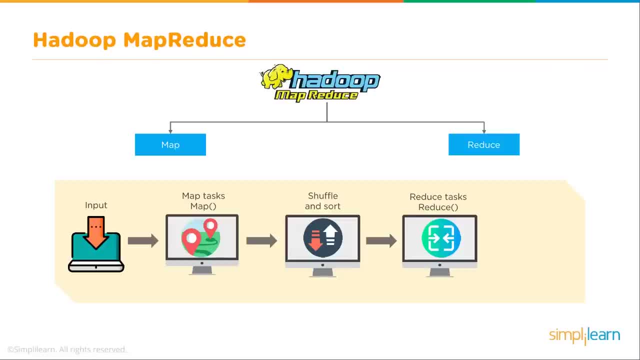 And each one of these is its own special piece of code or script, And finally we get the output. Again, we want an output that we, as a reader, can actually look at and understand, Whether it's a graph, word count, weight on each document. 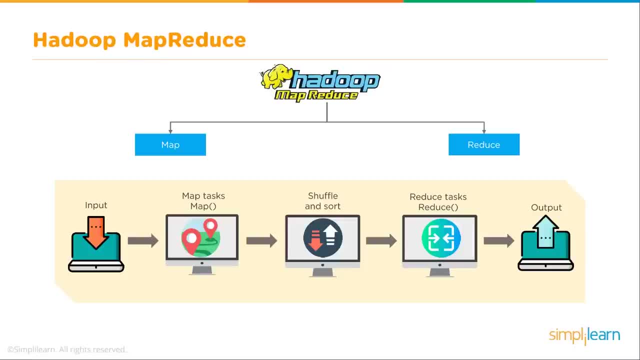 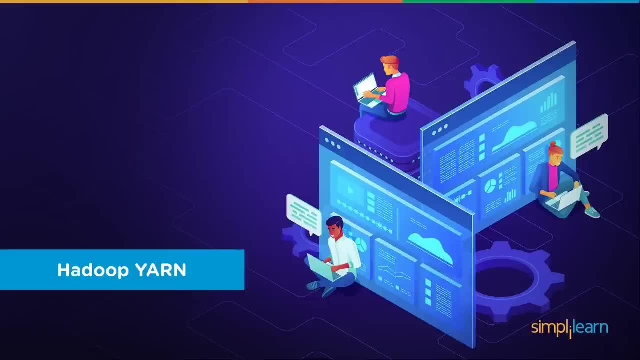 So we look at the whole Hadoop, map reduce, Think, map reduce, And the shuffle happens in the middle because it's just part of Hadoop, It's just part of getting to the reduce. So what about yarn? Hadoop yarn- This is the glue that holds it all together. 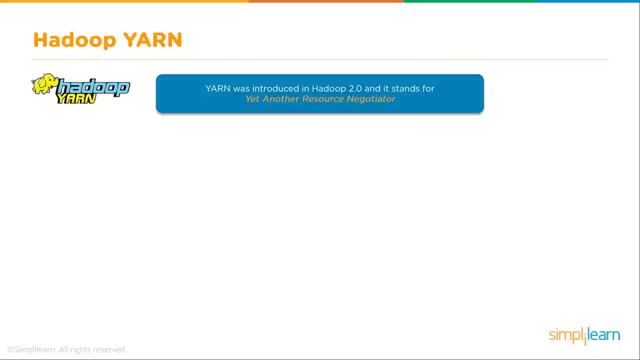 Yarn was introduced in Hadoop 2.0. And it stands for yet another resource negotiator And when yarn came out And they put that out in version 2.0. It was like one of the biggest jumps in Hadoop. 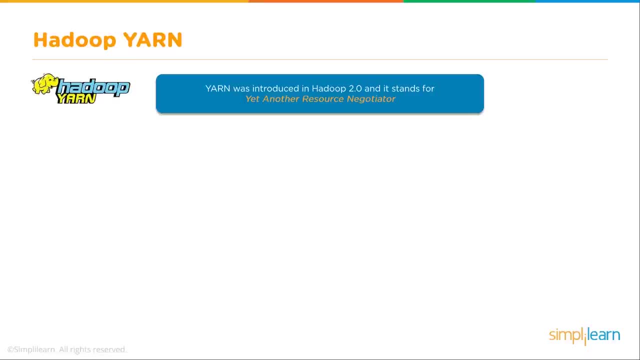 As far as it being really deployable and used in big business. And so we talk about yarn. Yarn is cluster resource management layer of Hadoop. It schedules the jobs And it assigns the resources to running applications. So when you're running as an admin on this cluster, 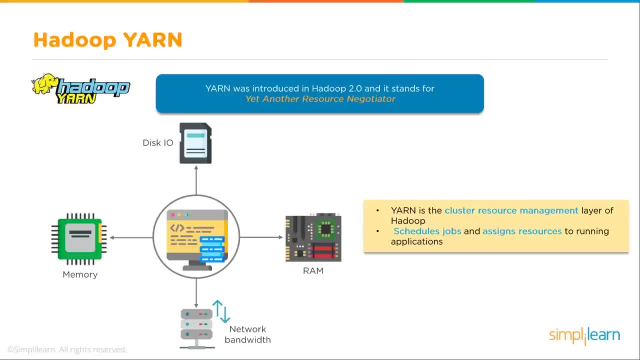 You want to know what's going on in the yarn. Where is it sending this information? Which computers are going down? Do you need to add another computer in? When you look at your disk in out, Your memory, Your RAM, Your network bandwidth. 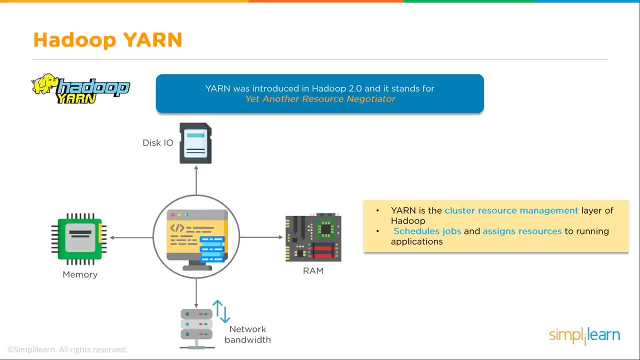 Do you need to put a new switch in? Do you need to add in? upgrade your computer so they have larger amounts of RAM? Maybe you're dealing with a huge data pool, So you need more hard disk drive on each of your computers. 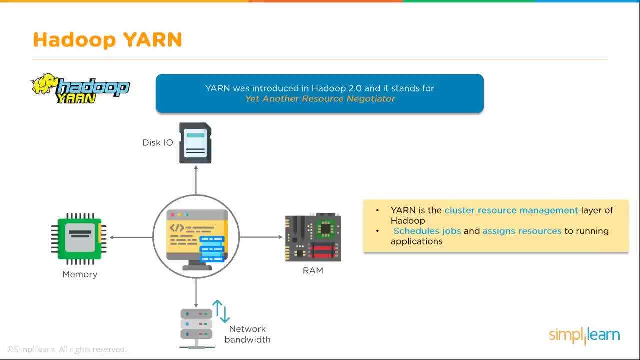 All these things are important. That's all part of the admin side, And so understanding how the yarn works Is so essential to being able to know what hardware to buy And how to configure it. When we look at the yarn architecture, We again have our client. 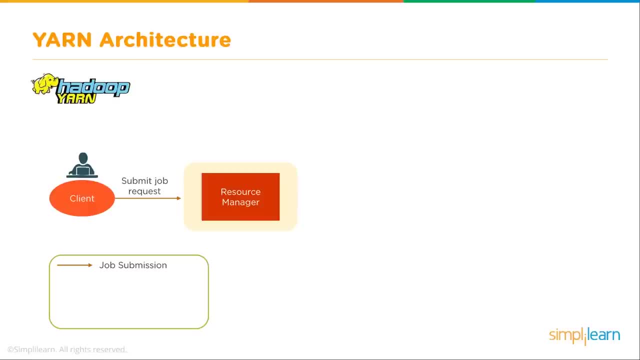 This would be your admin, Or well, it's actually the programmer sends it in. there Could be the admin who's monitoring the system And then when the yarn, The submit job request goes in And that goes into the resource manager. And once it goes into the resource manager, 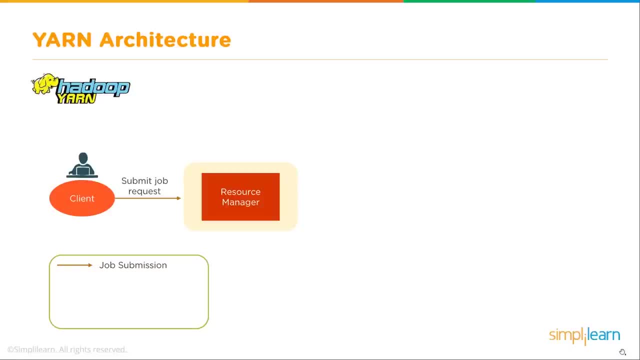 Then you get a job submission. Now the client usually is the programmer making the request, And so the admin wants to know: Hey, if that request doesn't come back Or the client is, you know, your boss's boss Is not getting the information he needs. 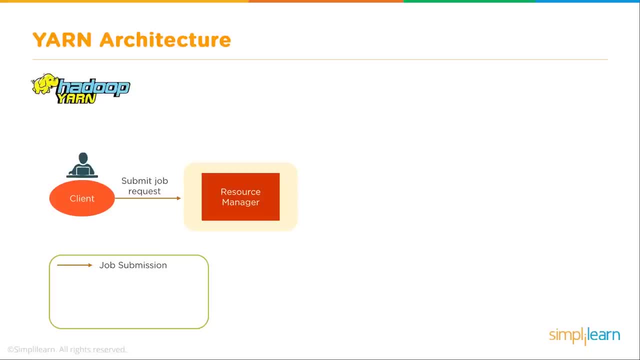 You need to be able to track down what's going on. Where did it stop? Did it stop in the resource manager? Did it stop in the job submission? And then, once we get into the job submission, You'll see we have our node manager. 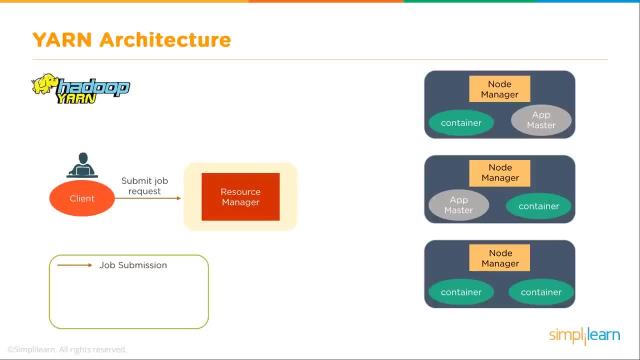 And it has its container and its app master, Another node manager, on the next computer App master container. So each of our nodes have these different aspects to them And our resource manager goes back and forth And they communicate with each other. So we have our job submission. 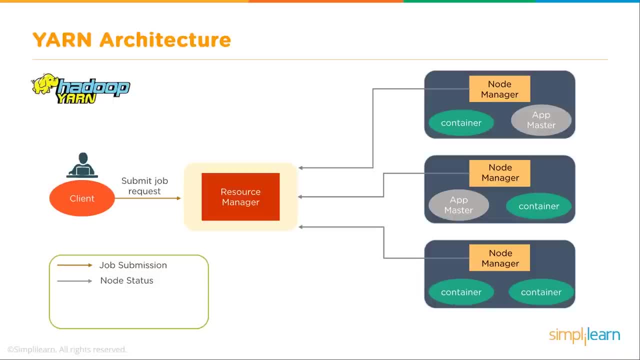 And then your node status- And that's part of the resource manager Is to track down the node status and know what's going on. And then, once that's all happened, Then we also are tracking down the map reduce status And we talk about Hadoop. 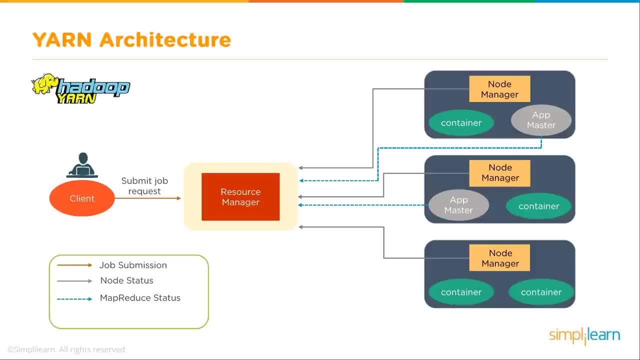 We're usually talking about batched jobs. That means we're going to deploy them And you'll get a note that says, Okay, my job is done In five minutes, Or in that one example, it took 17 hours For something that they thought would never even be computable on computers. 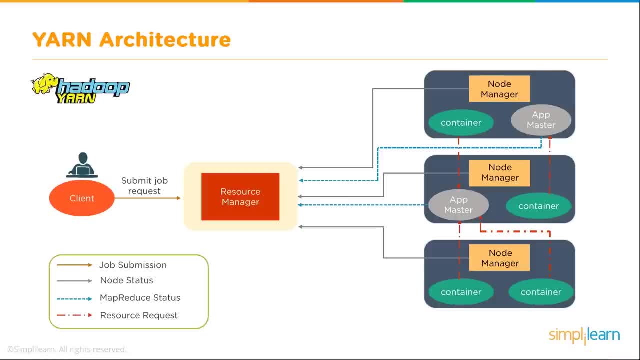 And then you have your resource request. Whatever was requested is sent back to the client. So they now have their information And so, as an admin on this, You really want to be aware Of what's going on in that resource manager. Usually you're looking up the node status. 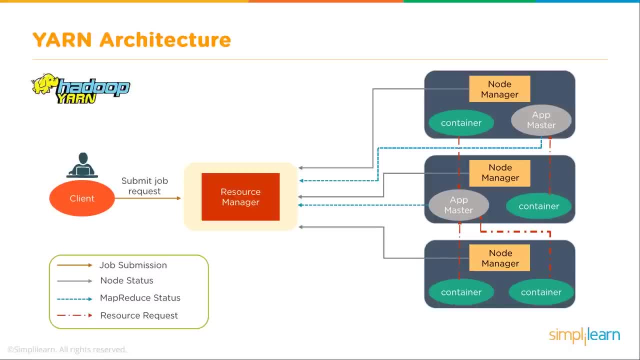 Do I have a bunch of nodes that are down? Do I have a rack that's down? You want to know the job submission. Maybe it got submitted And it was put in low priority or something, And the person's like: Why didn't I get my information back? 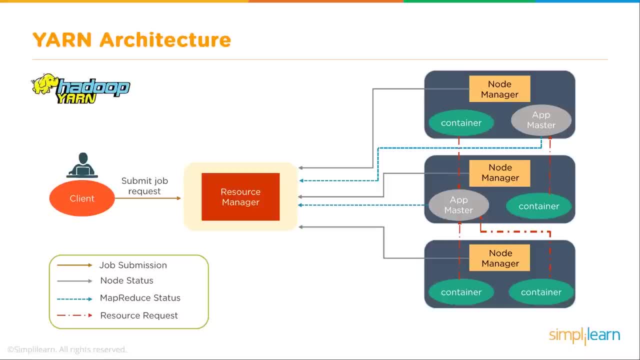 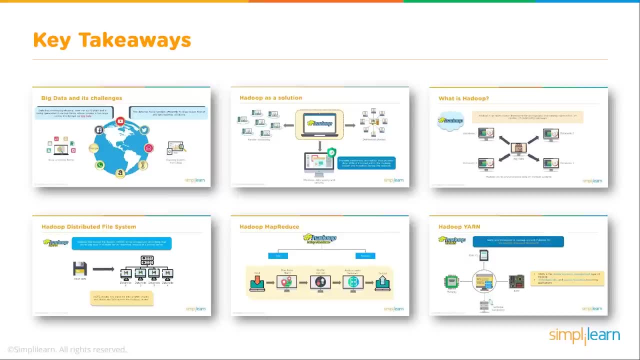 Why is this taking 20 minutes? And the same with the map: reduce status. Those both kind of go together. Let you know what's going on. So we covered a lot of basics. We covered in the key takeaways What is the challenges around big data. 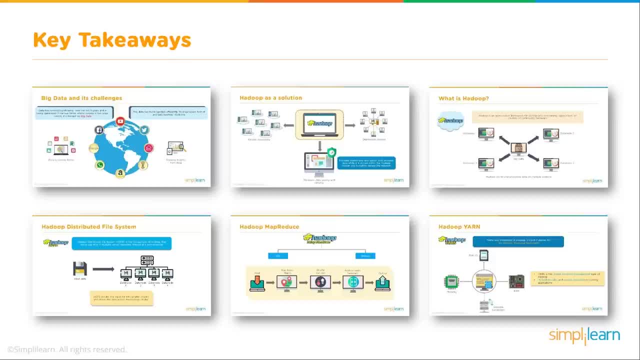 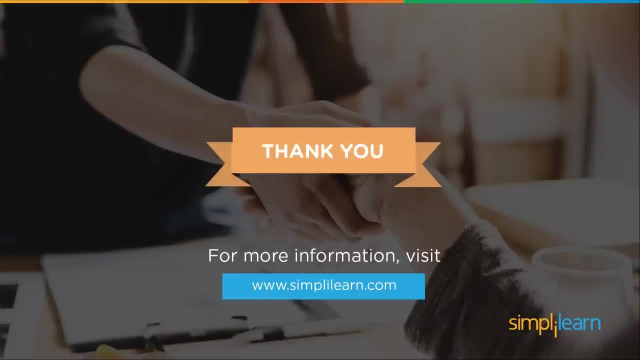 We looked at Hadoop as a solution And then we dug into what is Hadoop And the Hadoop distributed file system, The Hadoop map reduce And the Hadoop yarn- The three main components of Hadoop- To get more information. 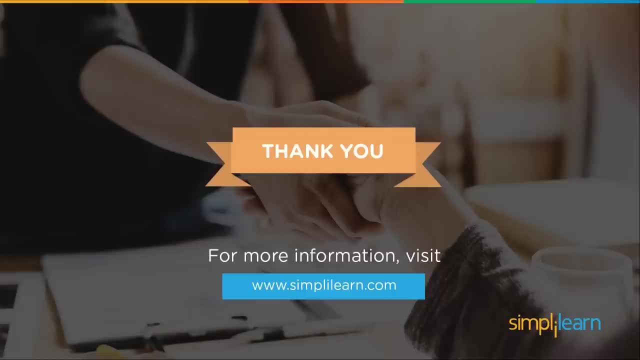 Visit wwwsimplylearncom. Get certified, Get ahead. We also manage the YouTube channel, So feel free to also post questions Down below in your YouTube channel And we'll try to have someone connect back up with you To answer those questions.